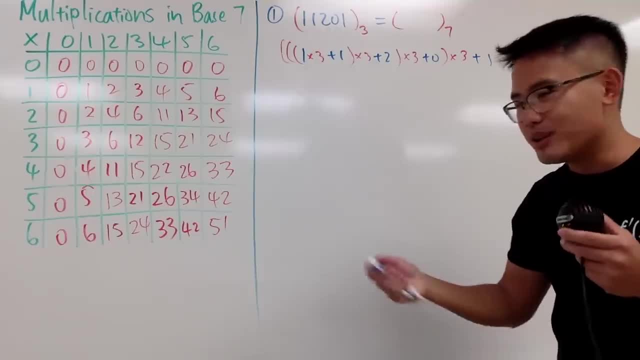 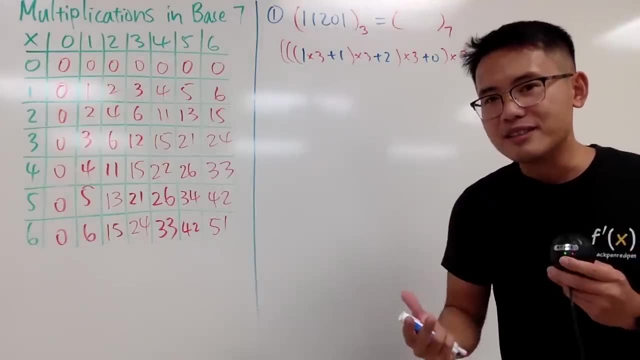 So it's the same thing. You pretty much just like factor out the 3s if you look at the usual expansion. But anyway, if you just work this out in the usual sense, you will get the answer in the usual sense, namely base 10.. 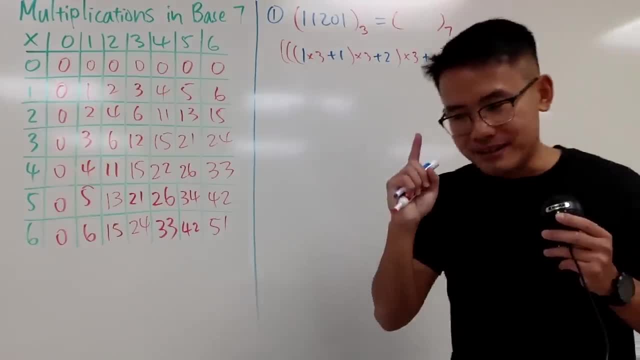 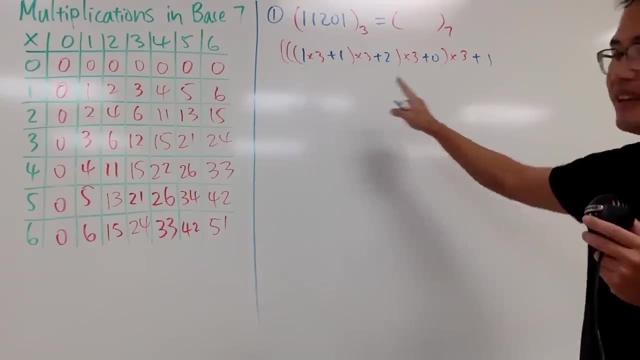 But if you do all the computation in base 7, the answer in the end will be The answer in base 7, right? So we are going to think everything in base 7 from now on. Okay, so here we go. 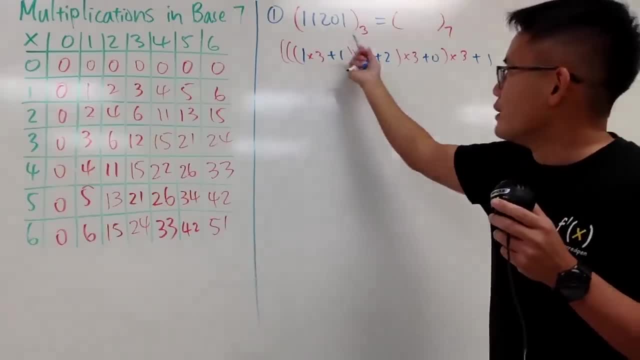 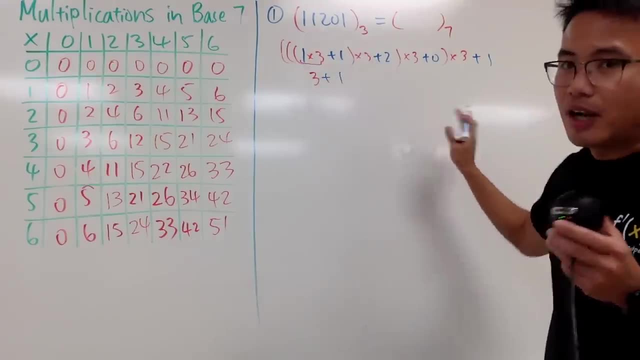 I am going to be looking at two numbers and operation at a time, of course. So here we go: 1 times 3, this is just 3,, okay, And then I will add 1. And I think this is how it should work. 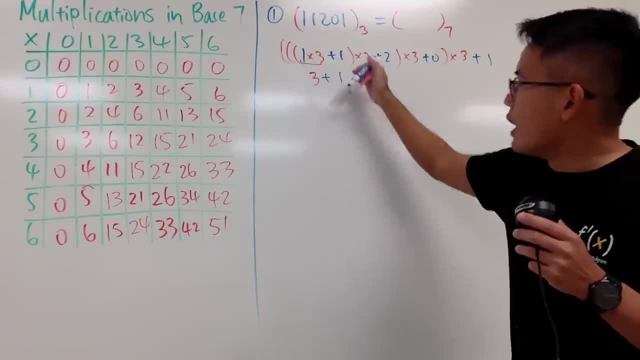 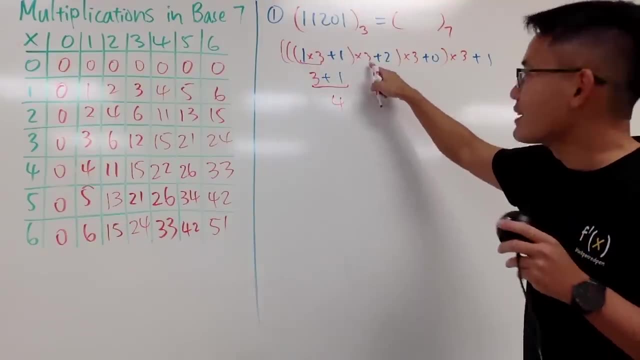 I'm not going to write down rest okay. So we have 3 plus 1.. And this is something we can do. So 3 plus 1 is 4.. Good, And next- This is the tricky part- We are going to multiply this by 3.. 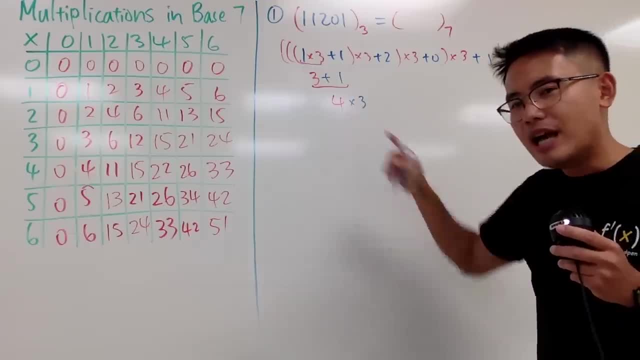 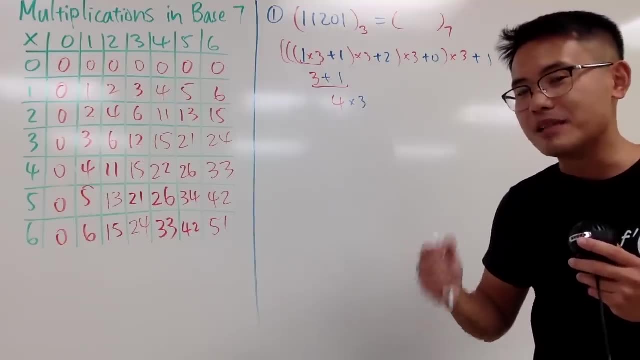 And now what is 4 times 3?? I know you want to say 12, but 12 in base 7 is what It's 1: 5. Because 12 is the same as 7 plus 5. So it's 1: 5.. 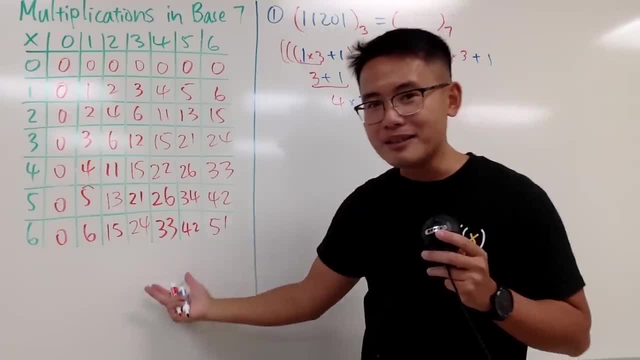 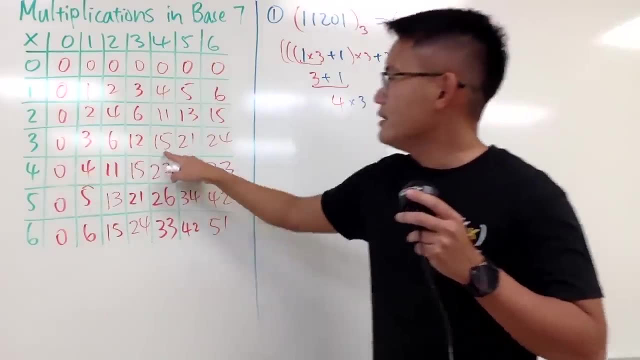 And this, right here, is why I tell you guys you should have the times table on the side in base 7.. So if you are going to do 4 times 3, you can look at 4 and 3.. You see, it is 1, 5.. 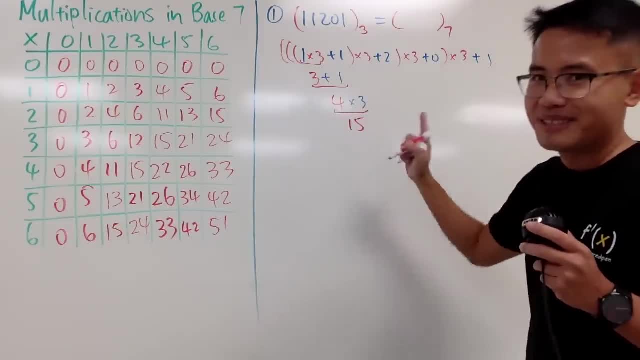 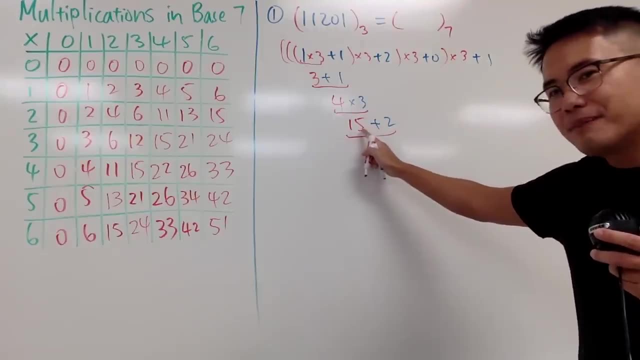 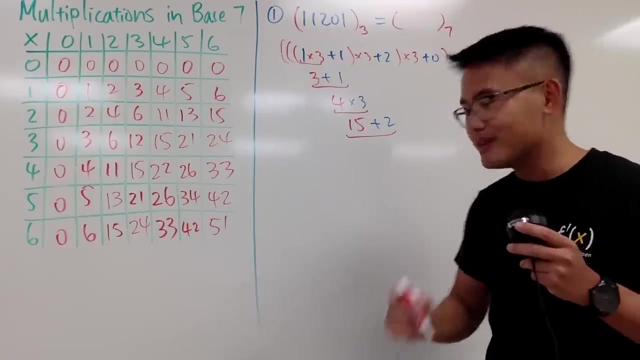 So 4 times 3 is 1, 5 in base 7.. And then we'll continue. We are going to add 2.. And you see 5 plus 2.. I know you guys want to say 7, but in the base 7 world you have to say 1- 0. 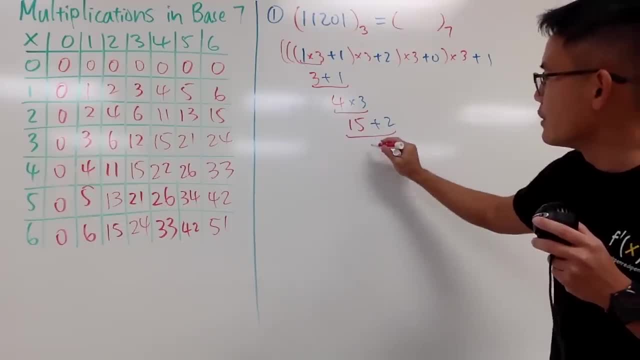 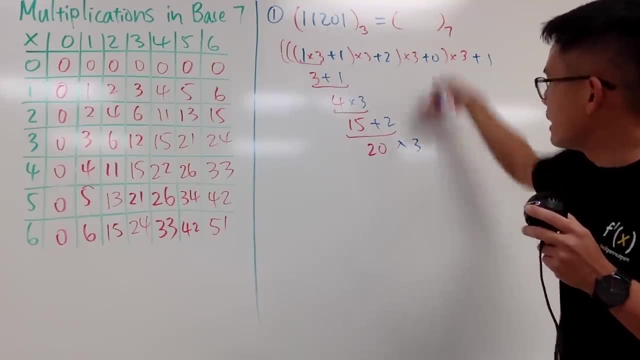 Once again, 5 plus 2 is 1: 0, and plus this 1,, so it's 2: 0, like this, And then we pretty much continue. Next, we are going to multiply by 3,, just line this up like this: 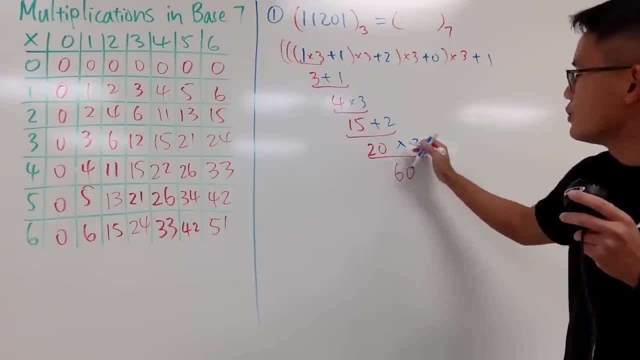 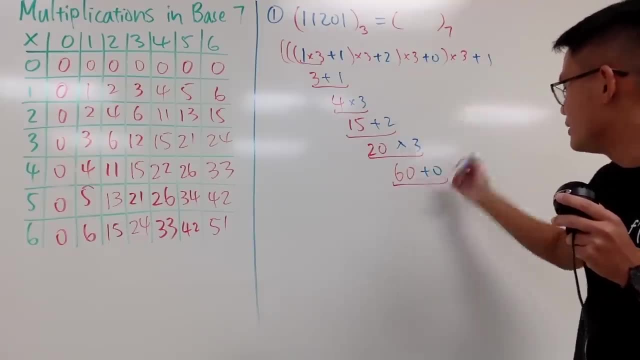 And then 2: 0 times 3 is just 6: 0, like 3 times 0 is 0, 3 times 2 is legitimately 6.. And then next I will just add 0,. so this is pretty easy. this is still 6: 0. 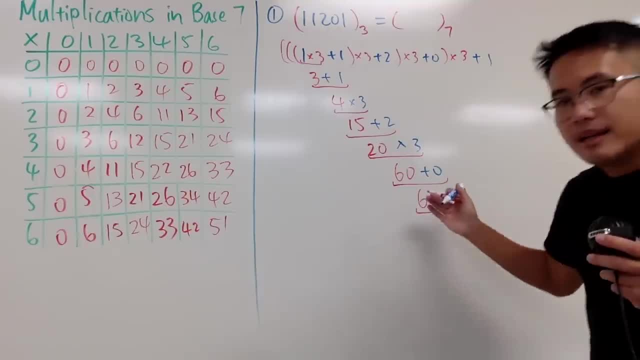 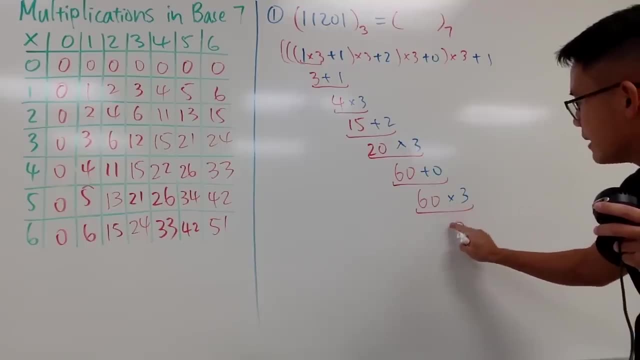 And then I will multiply by 3,, 6, 0 times 3, 3 times 0 is 0, and then 3 times 6 is. you can look at the times table on the side 3 and 6 right here. when you multiply you get 2, 4.. 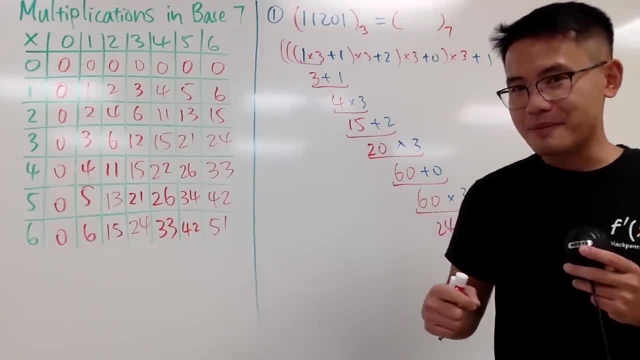 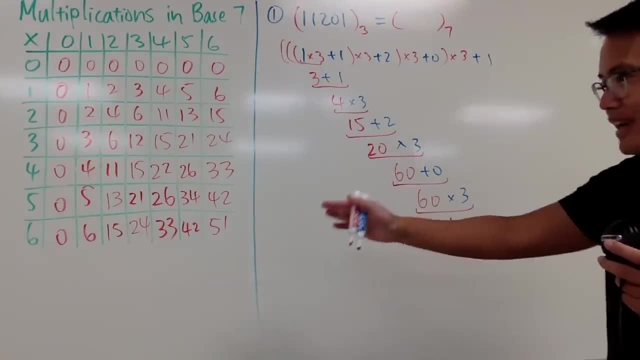 Why? Because 3 times 6 is 18.. 18 is the same as 14 plus 4, so you have to have 2 and 4 to get the 18.. 2 means 2 times 7 to the first power. that's how we get the 14, and then plus that 4.. 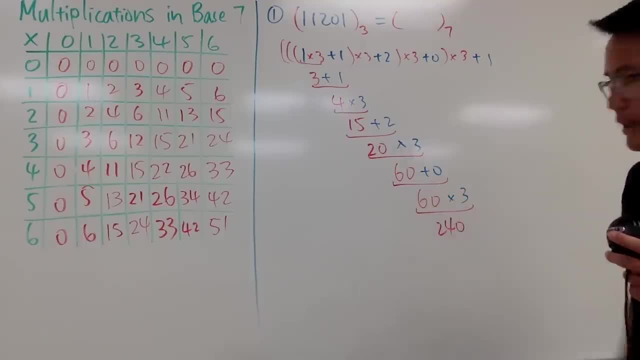 So, just as 3 times 6 is 2, 4, and then of course you have to add just 0. And in the end you just put down plus 1, and of course, when you combine all this, 2, 4, 1.. 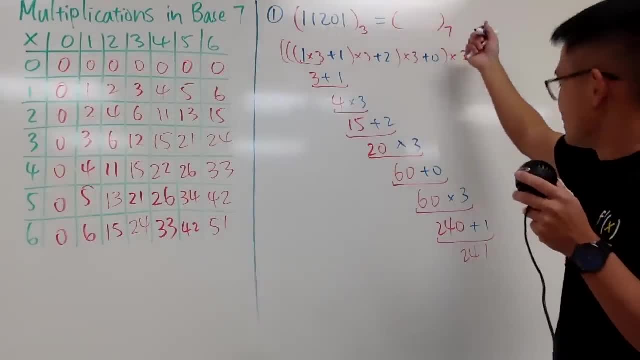 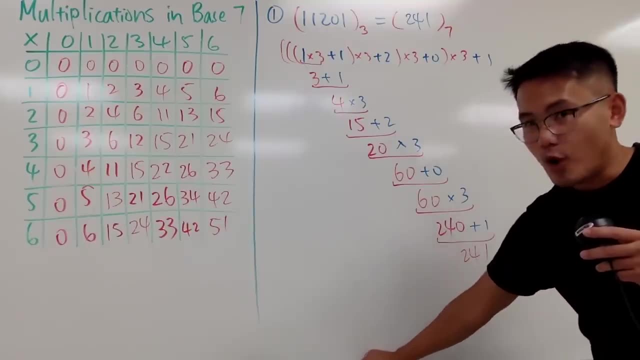 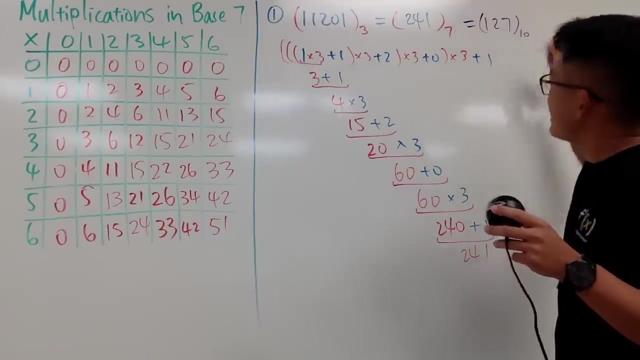 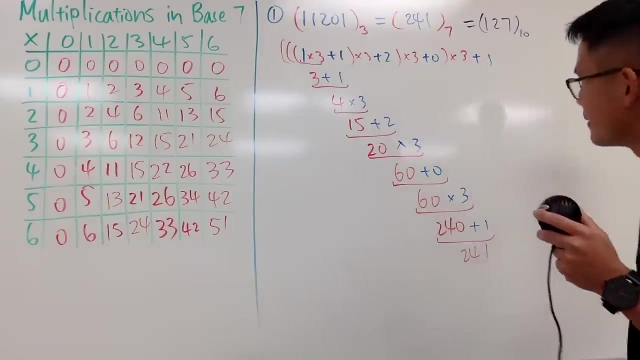 And here you have it. This number in base 7 is 2 4, 1, and that's it. And if you guys would like to know, both of this equal to the number 127 in base 10.. And now let's see how to go from a bigger base to a smaller base, right here. 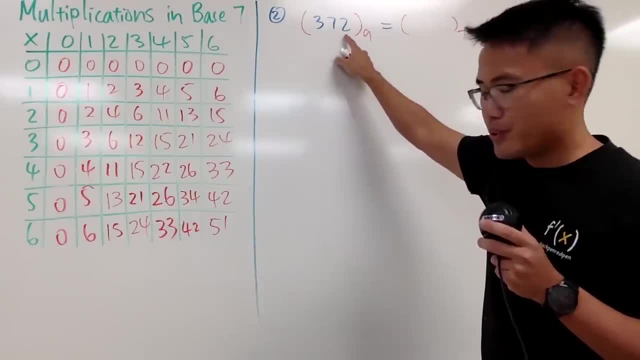 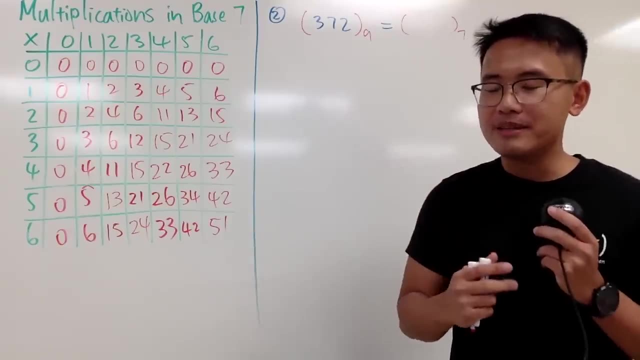 And I will show you guys this one: 3, 7, 2 in base 9, and we'll change that to base 7.. Okay, And when you go from a bigger base to a smaller base, you have some trouble. First of all, we still have to talk about how to expand this, but we have to do it really carefully. 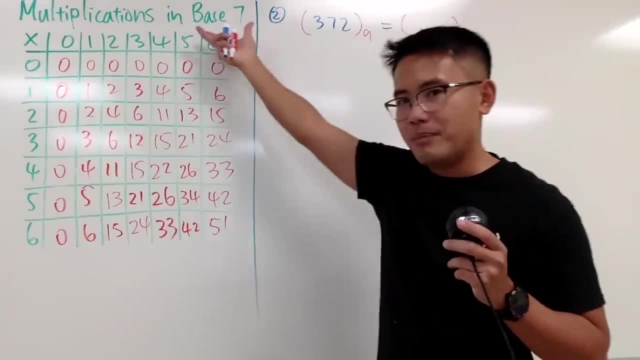 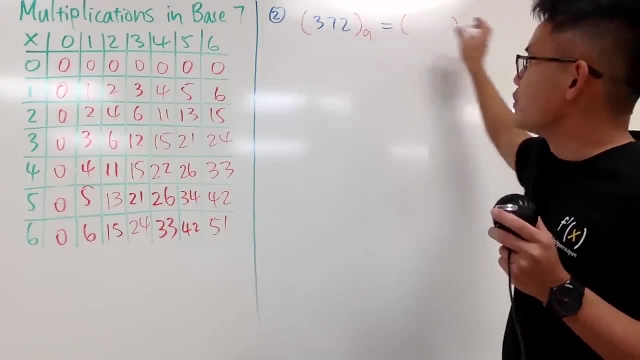 Because 7 is not allowed in the base 7 world. Likewise, 9 is also not allowed in the base 7 world. So when you go from a bigger base to a smaller base, this, right here, is a trouble. already. You have to know what is 9 in the base 7, okay. 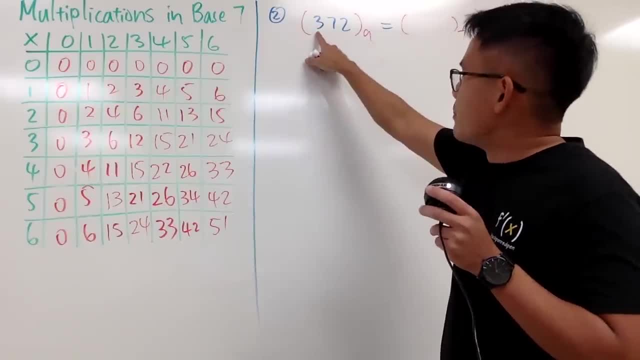 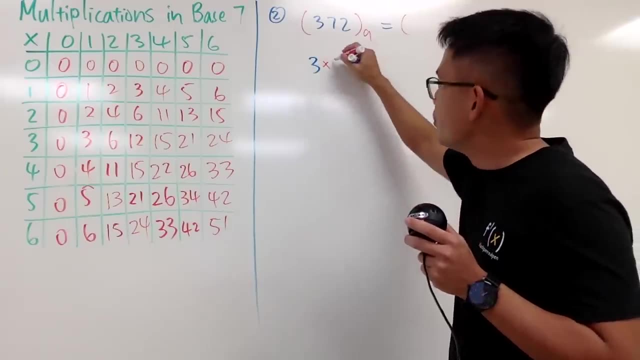 So let's do it carefully. I will start from the number from the bottom, From the left, which is this: 3 right here, And I will say: multiply by, I cannot put down 9.. I will have to put down 1, 2 right here. 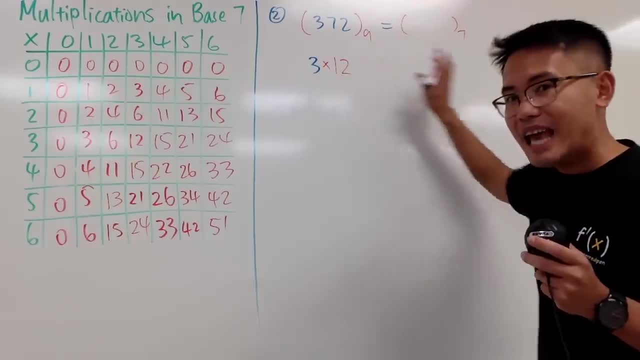 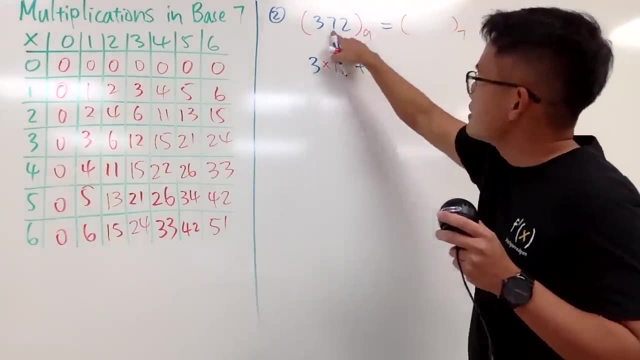 Because, remember, if you want to get to base 7, you have to think everything in base 7.. This right here is the 9 in base 7,. alright, And then I will add the next number, which is this 7.. 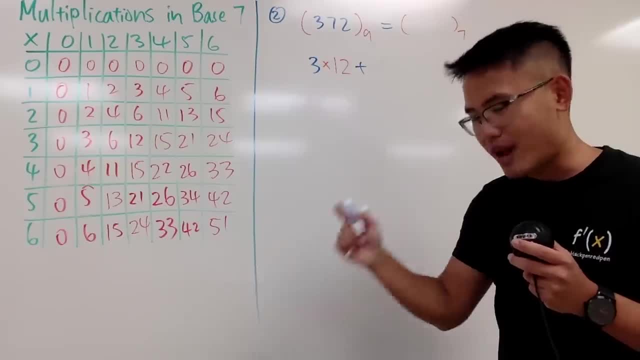 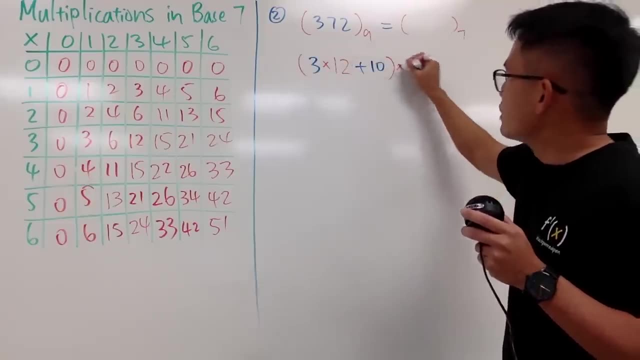 But 7 in the base 7 world is what 1: 0.. So I will actually put down 1: 0 here, And then we'll Put a parenthesis and then multiply by this in base 7, which is 1: 2.. 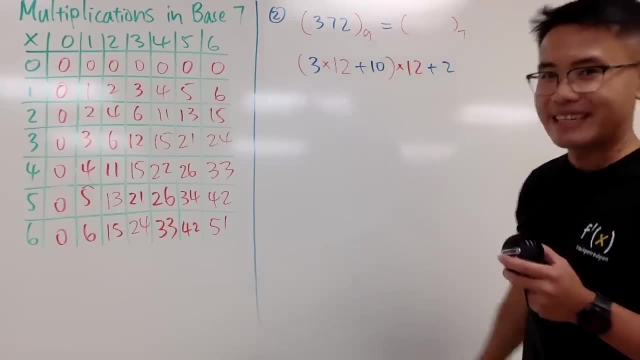 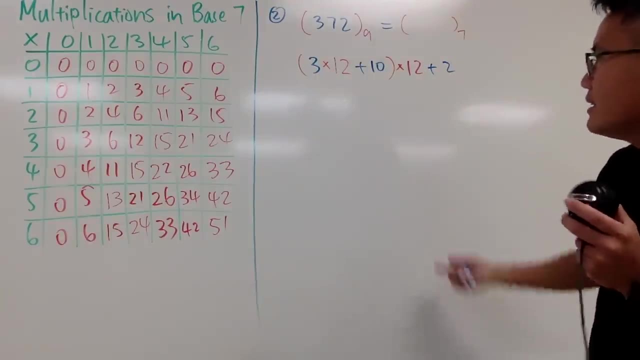 And then in the end, I will add 2, like this. So this is how I'm going to look at the expansion. alright, Because we are working everything in base 7 now And, just like earlier, I am just going to multiply this as how it is. 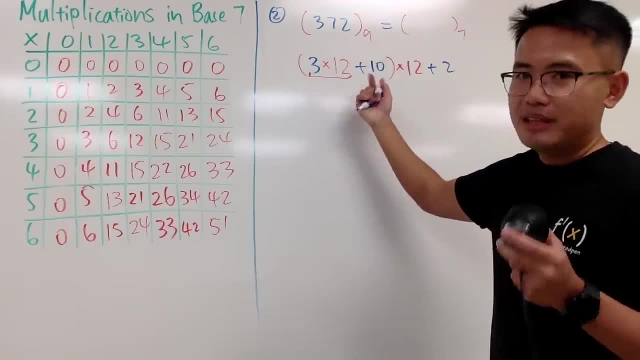 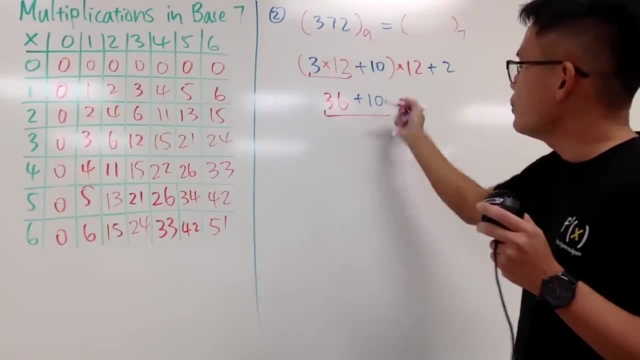 Okay, 3 times 1, 2 is just 3, 6.. This is okay, And then I'm going to add 1, 0 to it, And when I do that, This is just 4, 6, okay, 0 plus 6 is 6.. 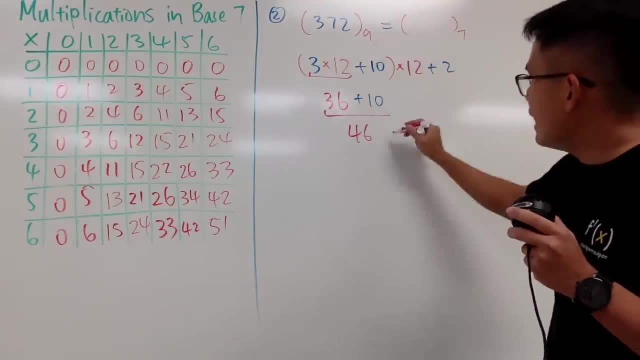 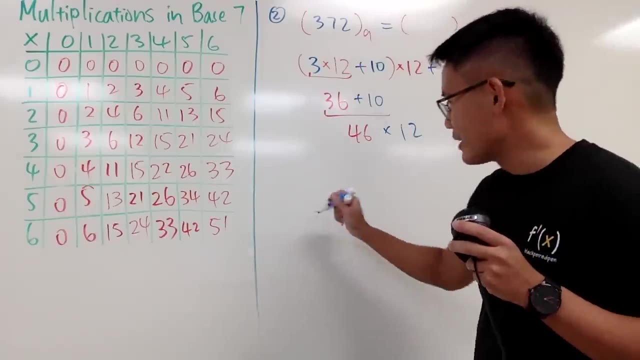 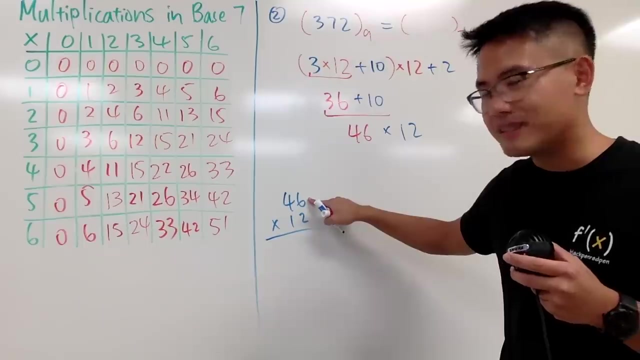 1 plus 3 is 4.. So far, so good. And then I will have to multiply by 1, 2 after that, And this right here is crazy, so let's do it on the side. Here we go: 2 times 6 in the base 7, I know it's 12 in the regular sense, but it's 1, 5 in base 7.. 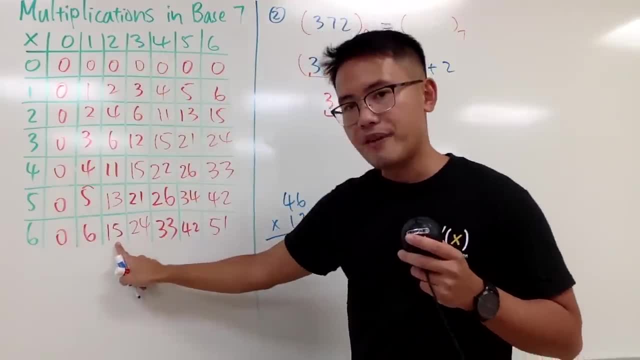 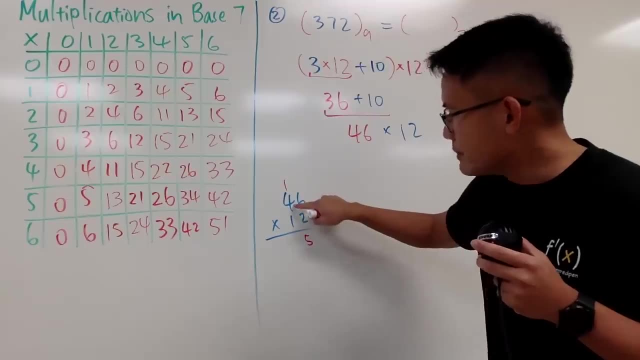 And, if you would like, you see, 2 times 6 is 1: 5.. So what you do is you put down the 5 right here And then you have the 1 5 like this right Next: 2 times 4 is 1: 1.. 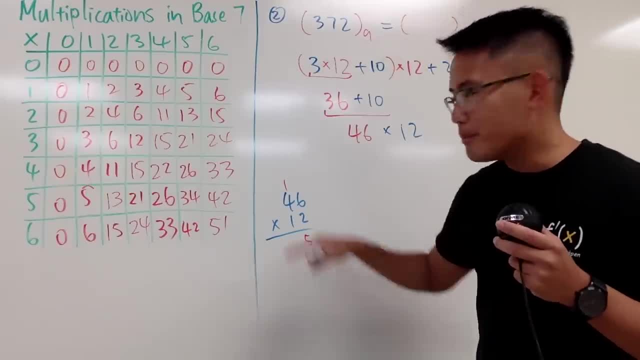 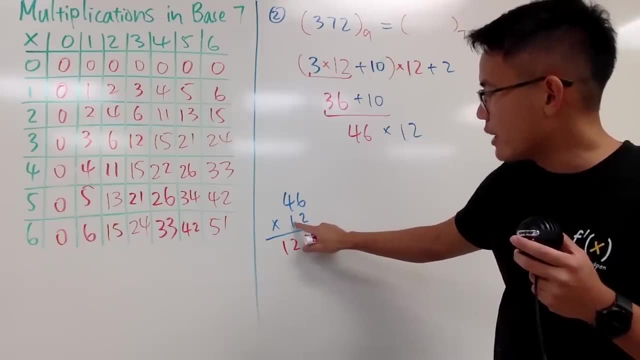 If you would like, 2 times 4 is 1, 1.. So 1, 1 plus this 1, you get 1, 2, okay, So this is it with the 2, right here and now we move on to this 1.. 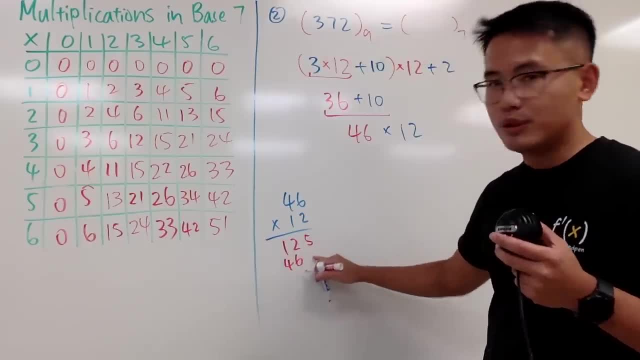 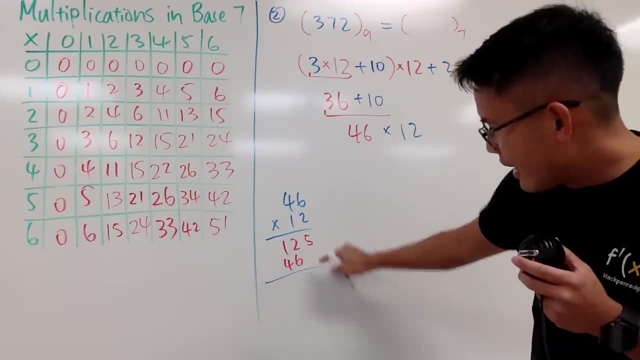 And 1 times. this is just all that, which is just 4, 6, like this. Of course, you leave a blank right here And then you are going to add them up in the base. 7 sense 5.. 5 and nothing is 5,. 2 and 6 is 1, 1.. 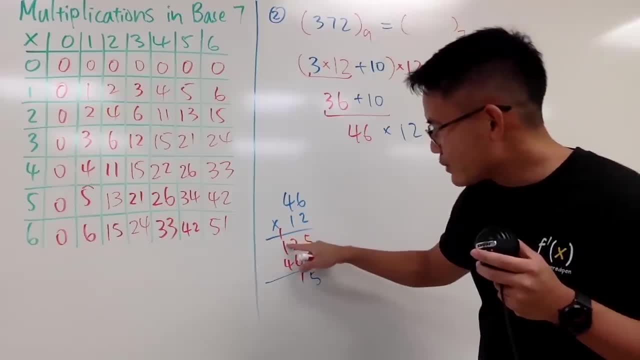 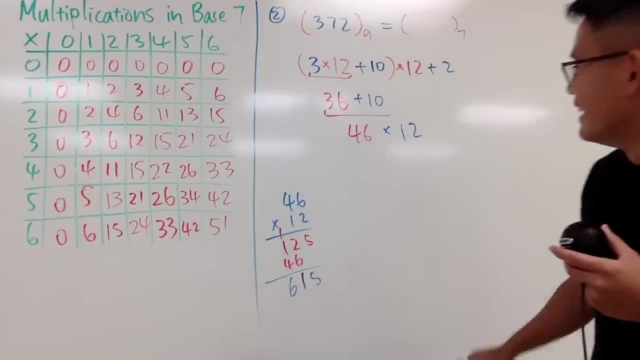 So 1, 1, okay, And then 1 plus 1 is 2, plus 4 is 6.. So you have 6, 1, 5, like this. Alright, so this right here. after you multiply it, you get 6, 1, 5.. 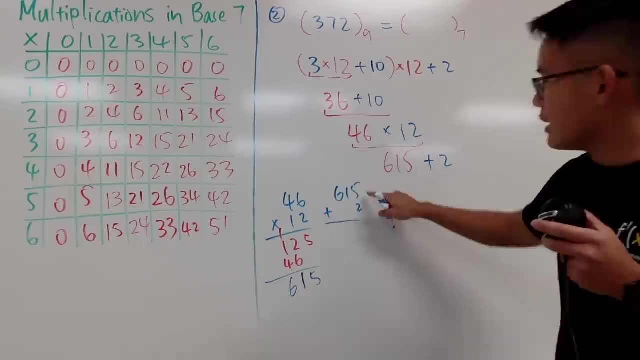 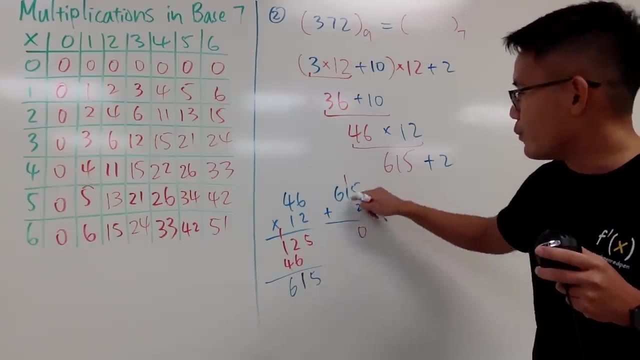 And then just one more. we are going to add 2 to it, 5 plus 2.. I know it's 7.. You have to say that's 1: 0. And then 1: 1 is just 2..